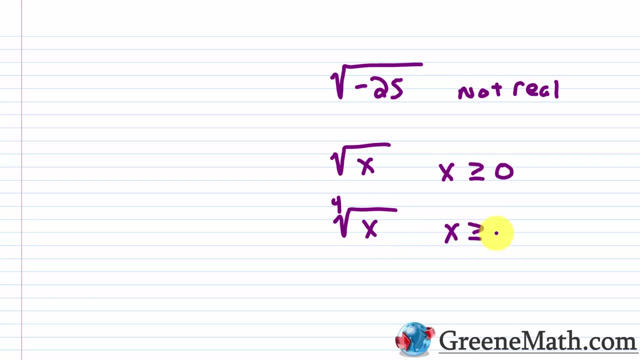 fourth root of x. well, again, x has to be greater than or equal to zero, Because, again, if you plug in a negative here, here, you can't do that right. You don't want the square root of a negative, you don't want the 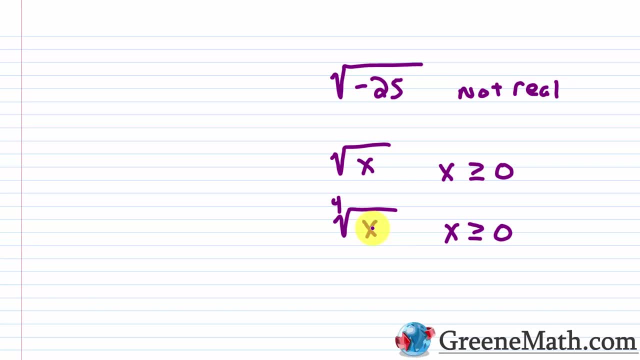 fourth root of a negative. you don't want the even root of a negative. Now, if you get something more complex, let's say you had the square root of something like x minus seven- well, here you need to make sure that this radicand ends up as a non negative value. So what you do is you take your 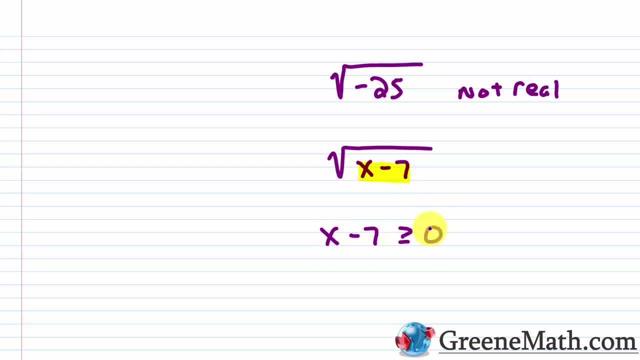 expression and you're going to set it as greater than or equal to zero. this is going to give you any domain restrictions that you would have. you're going to find the allowable values for x by doing this, So I'm going to add seven to both sides of the inequality And 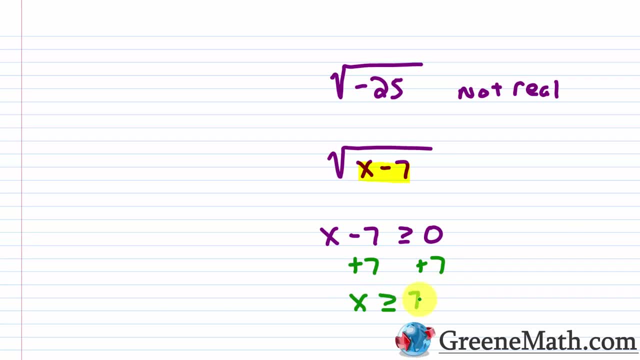 I'm going to find that x must be greater than or equal to seven. okay. So if x is seven, we're okay, because seven minus seven is zero, square root of zero, that's fine, that's just zero. But if x is, 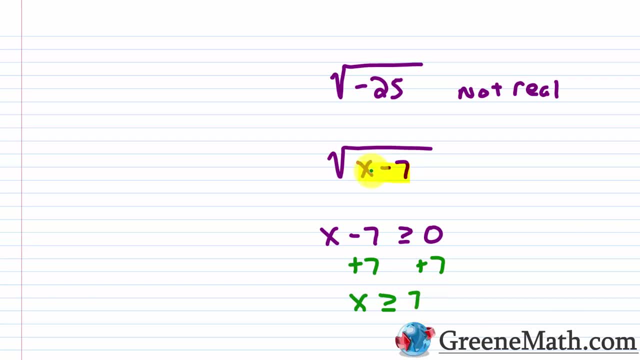 something less than seven, well then we have a problem, right? If I plugged in six there, six minus seven would be negative. one square root of negative one again is not real. So when you're working with again square roots, fourth roots, six roots, you know so, on and so forth, you need 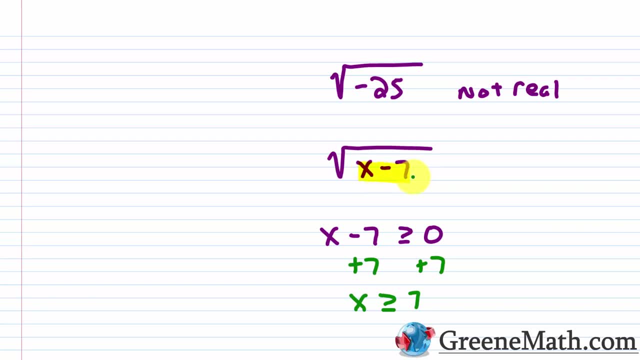 to make sure that if it's an expression under there with a variable you set, that guy is greater than or equal to zero and you solve it And that's going to give you any domain restrictions that you would have Again. for this example, we found that x must be greater than or equal to seven. 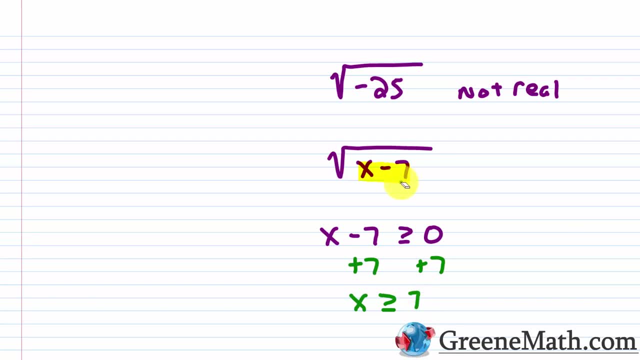 Now if we're working with a radical with an odd index, you don't have this issue right. We know this is a real number. this is negative two right, Because I can raise a negative number to an odd power and get a negative okay. So the cube root of negative eight is negative two. 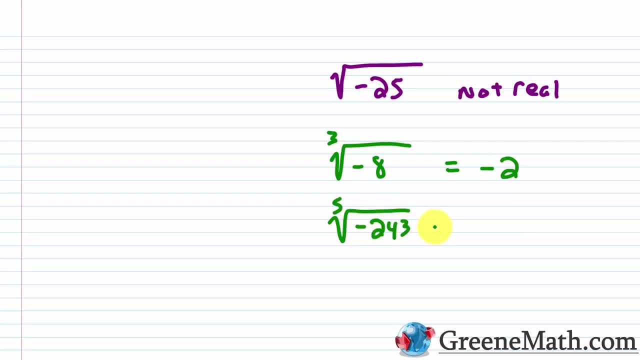 or the fifth root of, let's say, negative 243 would be negative three, right? Because negative three to the fifth power is negative 243.. So if I got something like, let's say, the cube root of x, this is valid for any real number, right? So I can plug in anything for. 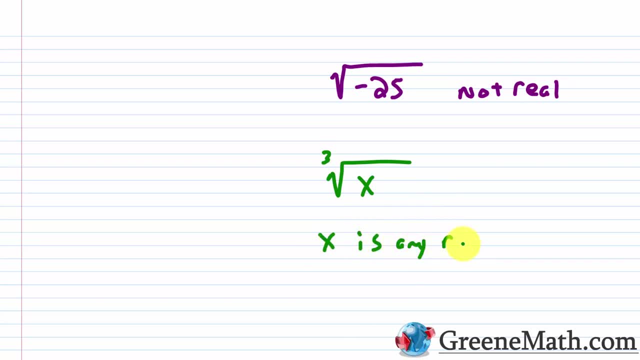 x. You can say x is any real number, okay, So with an odd index you don't have those restrictions. All right, let's jump in and look at a problem. So we have that three times the square root of x plus three plus 13 is greater than or equal to 16.. So the first thing I would 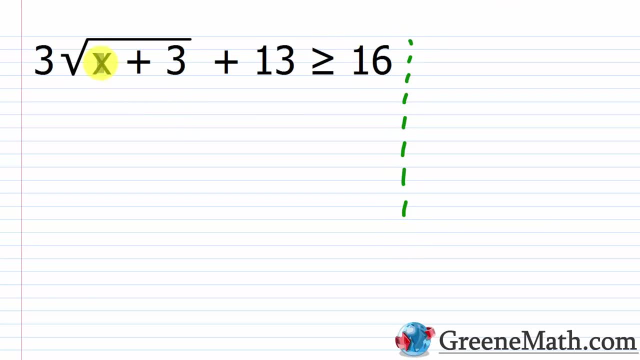 do with this type of problem is find the domain restriction. So we would take this expression here for our radicand, this x plus three, and we would say it has to be greater than or equal to zero. right? This is what we're going to accept as values for x. So let's subtract three away from both sides. 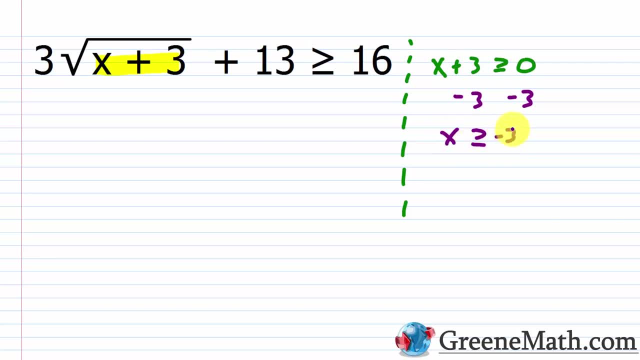 of inequality, We're going to find that x must be greater than or equal to negative three. Again, that makes sense because if I plug in a negative three here, negative three plus three is zero. So you're good there, right, Square root of zero. you're fine, That's zero If you plug in. 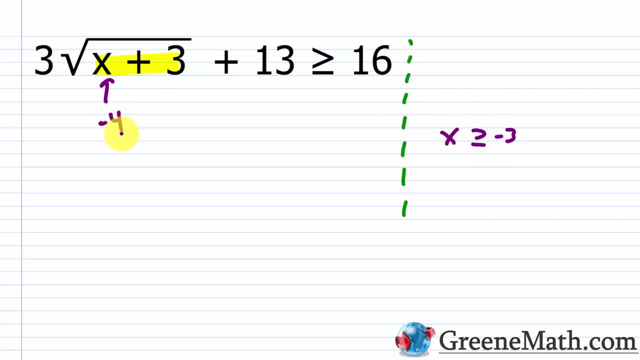 something less, though you've got a problem If you plugged in a negative four. negative four plus three is negative one. Square root of negative one again is not real, So let's state this again as our domain restriction. Officially, what we would do is look at aacceptanceым, breathing in. 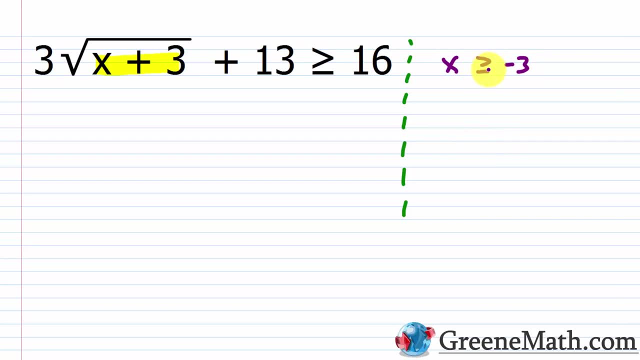 breathing out. Here's a picture today from a분 break, just to show what we could do: 17.. So what we're going to do, we're going to look at some things in the names solved, including our equation. So right now, what's going on is we're going to our equation and 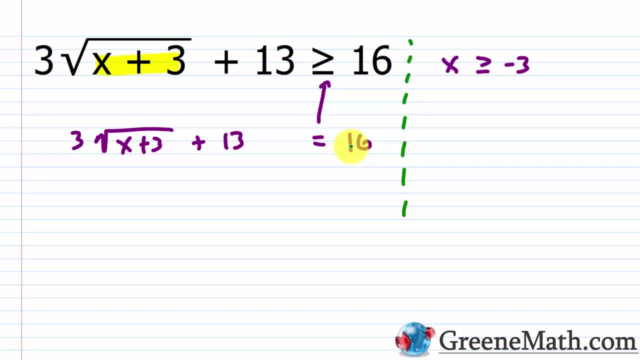 solve for that equation. So the first thing we're going to do is do an equation and then we're going to solve for our equation, And then I'm going to look at my number line and I'm going to test each side of the boundary. 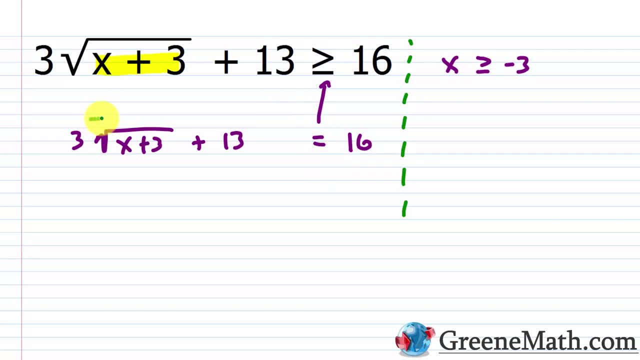 So how do we solve this? We know that our goal is to isolate the radical to start. So I'm going to subtract 13 away from each side of the equation, and we know that this is going to cancel. We'll have 3 times. the square root of x plus 3 is equal to 16 minus 13 is 3.. 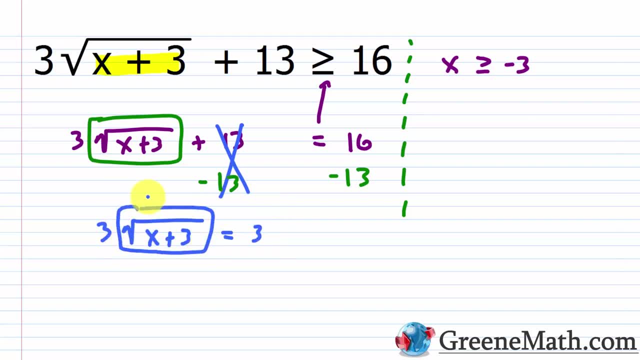 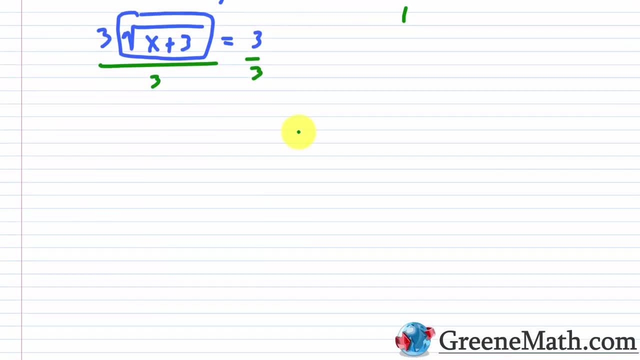 So now to isolate the radical, all I want to do is divide both sides of the equation by 3.. And that's going to give me what? Let me kind of scroll down and get some room going. That's going to give me that the square root of x plus 3 is equal to 1.. 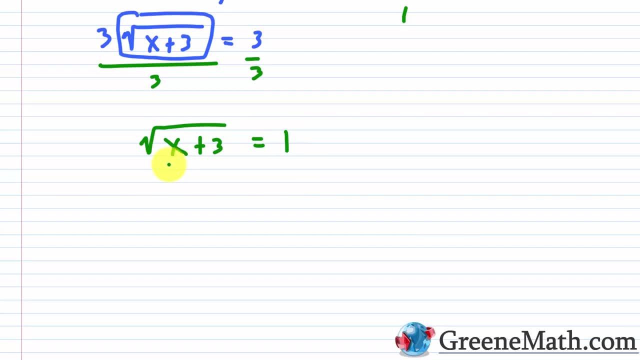 Now that I have my radical isolated, I can square both sides to get rid of it. So I'm going to square this side and I'm going to square this side. Now, remember, when you square both sides of an equation, you might end up with extraneous solutions. 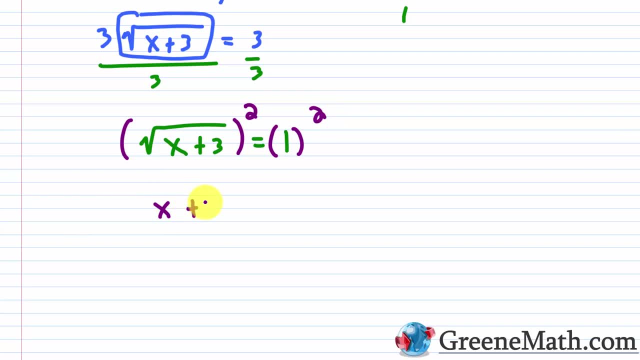 So we've got to make sure we check. So this guy is going to end up as: x plus 3 is equal to 1.. So to solve this guy, I subtract 3 away from each side. So I subtract 3 away from each side of the equation and I end up with x is equal to negative 2.. 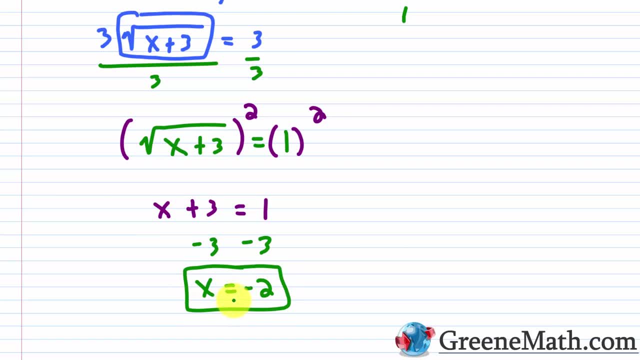 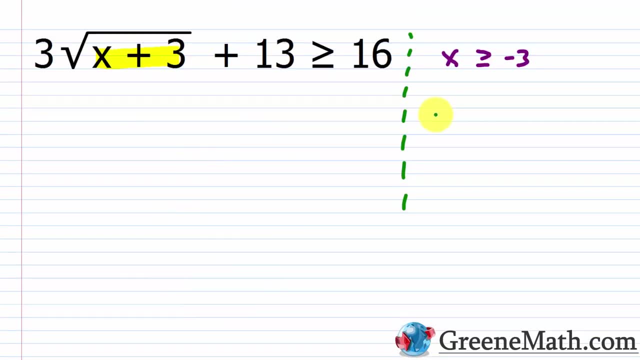 So this is my boundary. okay, If I plugged in a negative 2 for x, the left side is going to end up as 16.. So let's see that real quick. So let me write this down here, as my boundary x is equal to negative 2.. 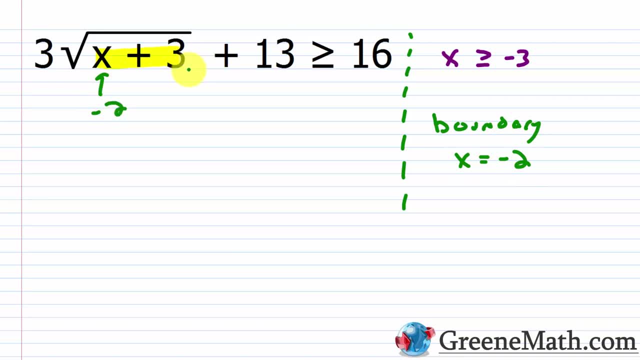 So again, if I plug that in here, negative 2 plus 3 is 1.. Square root of 1 is 1.. So you basically have 3 times 1,, which is 3, plus 13,, which is 16.. 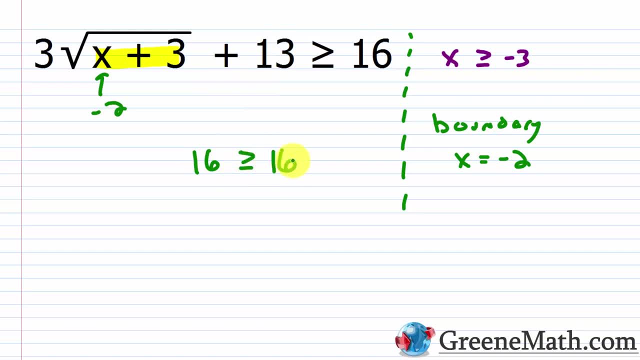 So you would get that 16 is greater than or equal to 16.. Again, if this was an equation, you'd see that you have a true statement, right? So we know that this solution here is not extraneous. okay, But consider the fact that you get: 16 is greater than or equal to 16.. 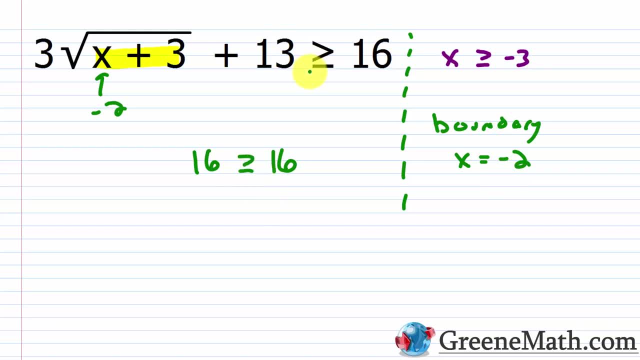 So we know that a value of negative 2 works as a solution for the inequality, so it's going to be included. Now what you need to do is test values on each side of negative 2 to see if they work All right. so we come down to the number line and essentially, we know that. 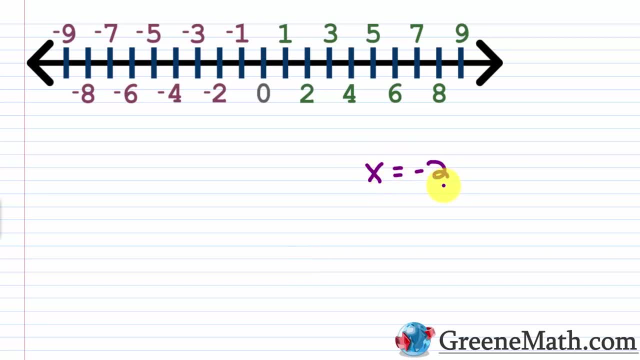 x equals negative 2 is our boundary. okay, Let me just label this for the first problem. So this is our boundary. Again, some people call them critical values, critical points, whatever term you want to use. So at negative 2, I'm just going to put a vertical line here. 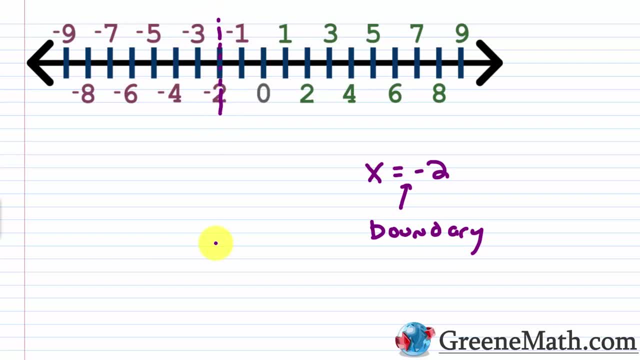 So to the left of negative 2, we have values that are less than negative 2.. To the right of negative 2, we have values that are greater than negative 2.. So we want to see what's going to work in the original inequality. 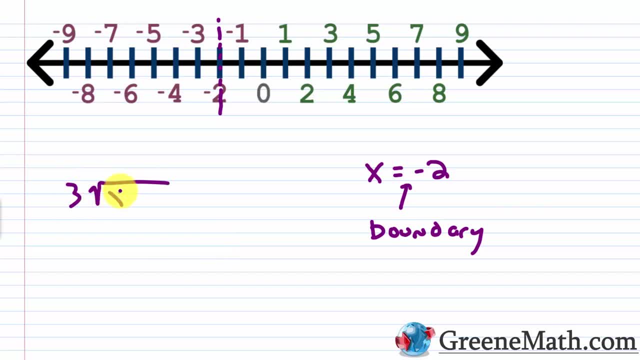 So we have 3 times the square root of x plus 3.. Then plus 13 is greater than or equal to 16.. Now this is subject to our constraint right, Our domain restriction, that specifically told us that x had to be greater than or equal to negative 3, okay. 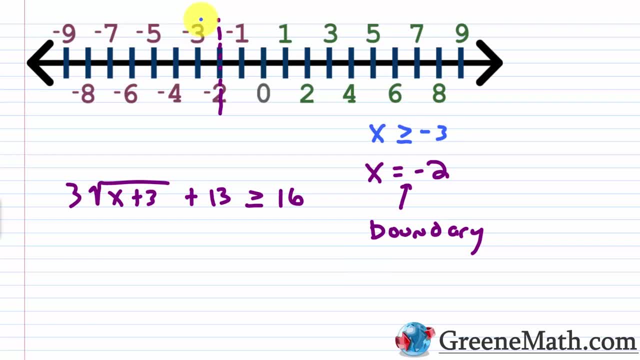 So really you could make another interval here if you wanted to. You don't have to, but you could make another one just to visibly say that, hey, anything to the left of negative 3 is not going to work. So if it shows up as a solution, you've got to reject it. 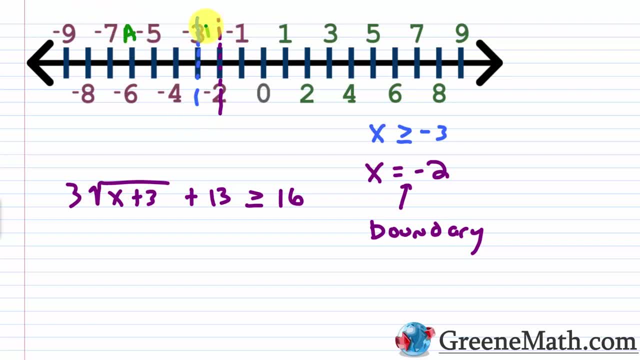 So I'm just going to label. I'm going to label this as interval A, I'm going to label this as interval B And I'll label this as interval C, just to keep track of what's going on. So what we're going to do here is we're going to test a value in interval B and C only. 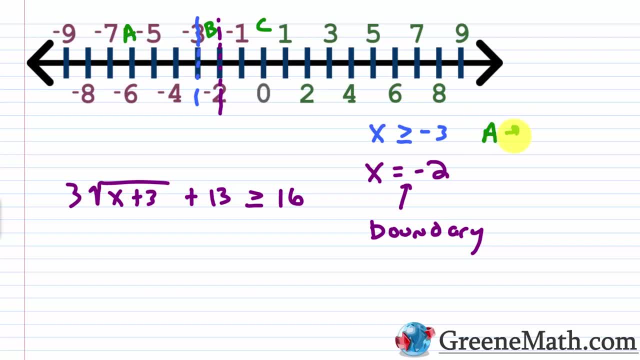 We don't need to test stuff in interval A. That's an automatic rejection zone. We'll put a false there, an F for that, because again it violates the domain. So between negative 2 and negative 3, so I'm going to pick a value of negative 2.75.. 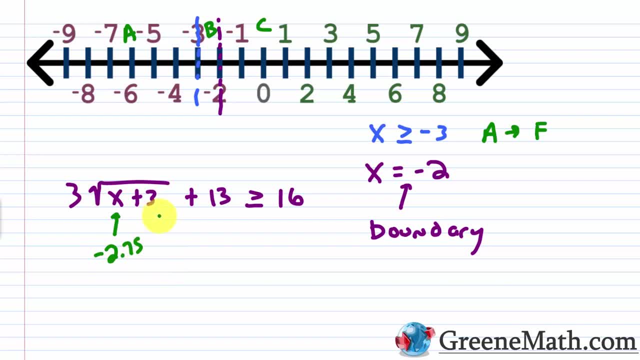 So negative 2.75.. Plus 3 would be 0.25.. So I would have 3 times the square root of 0.25. plus 13 is greater than or equal to 16.. So what's the square root of 0.25, or what's the square root of 1.4?? 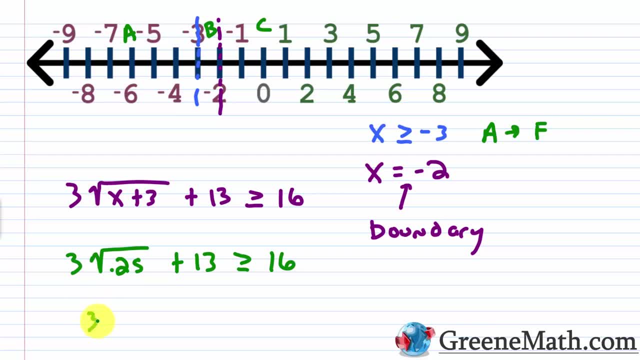 Well, it's going to be 1.5. So this would be 3 times 0.5, or 3 times 1.5, plus 13 is greater than or equal to 16.. And again, 3 times 1.5 is just 3 halves. 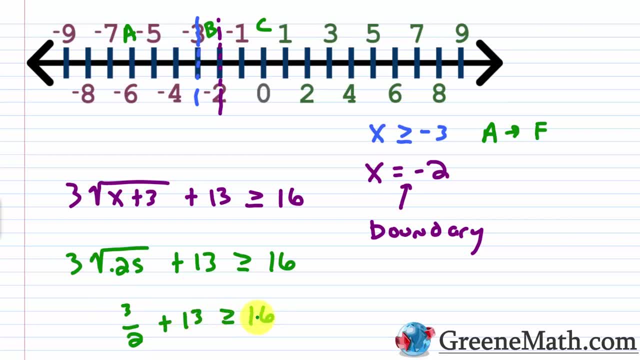 So you'd have 3 halves plus 13 is greater than or equal to 16.. Without going through and getting a combination, you'd have a common denominator and all that stuff. You can see that's not going to work right. This is basically going to be 13 plus 1.5, which is 14.5.. 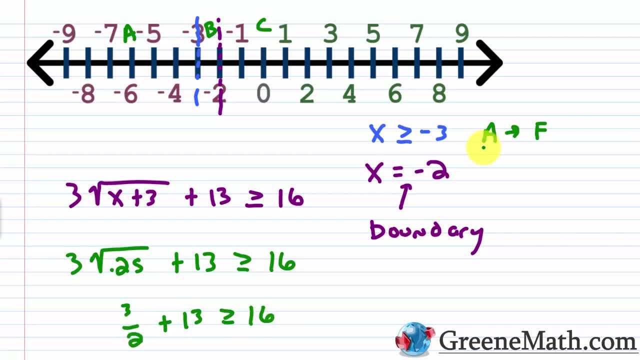 That's not greater than 16, and that's not equal to 16.. So things in interval B are not going to work. We'll put this as false also. So what about things in interval C? What about things that are greater than negative 2?? 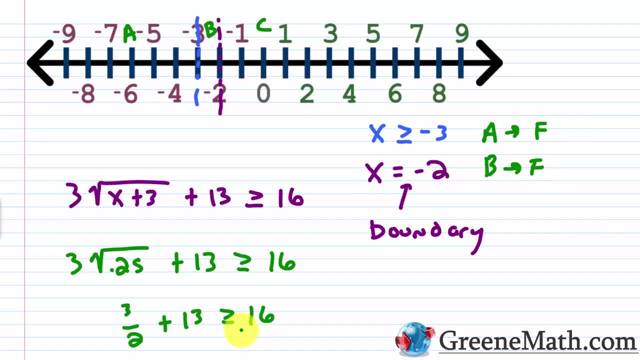 We already know that negative 2 works because it's a non-strict inequality, and we tested it earlier. But what about things that are greater than negative 2? Does that work? So for interval C, Well, let's go ahead and try. 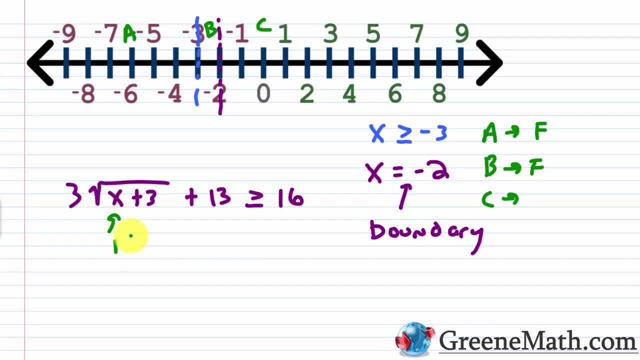 To make this easy on ourselves: a value of 1.. So we'll plug that in: 1 plus 3 is 4.. Square root of 4 is 2.. So you'd have 3 times 2, which is 6, plus 13,, which is 19.. 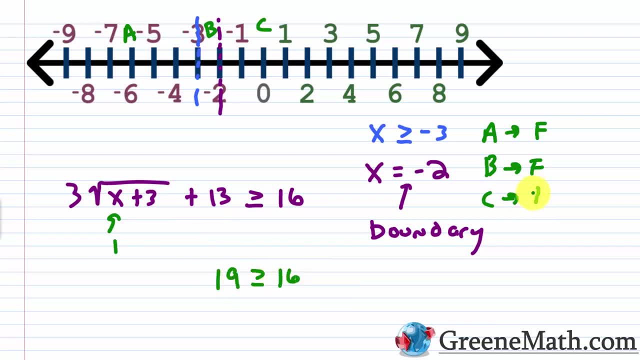 So you'd have: 19 is greater than or equal to 16, which is true. So things in interval C will work. So that's where we're going to have our solution region. So interval C is anything greater than negative 2.. 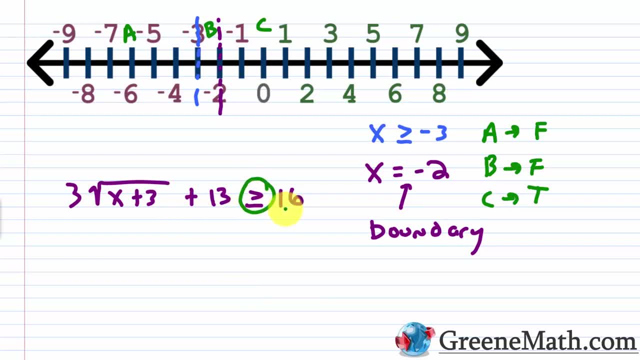 And again, because this is a non-strict inequality here and we tested it right- If we plug in a value of negative 2, negative 2 gives us a value of 16 on the left. we'd have 16 on the right. 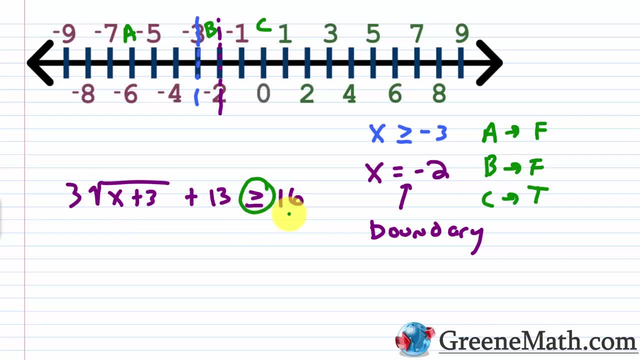 16 is greater than or equal to 16.. That's true, right. So negative 2 does work. So we would say that our solution here is: x is greater than or equal to negative 2.. And the great thing here is that it doesn't violate our domain right. 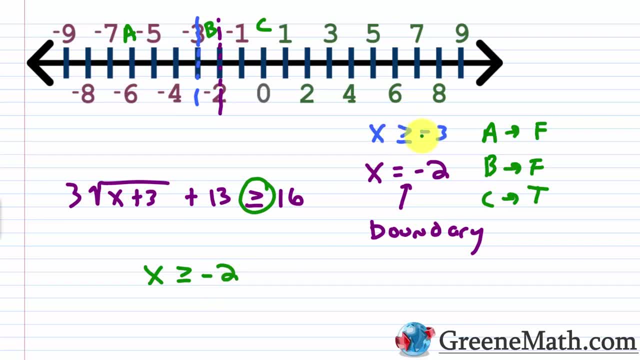 Our domain says that it has to be greater than or equal to negative 3.. We're greater than or equal to negative 2. So we're basically good to go. So in interval notation we put a bracket, a negative 2, a comma. 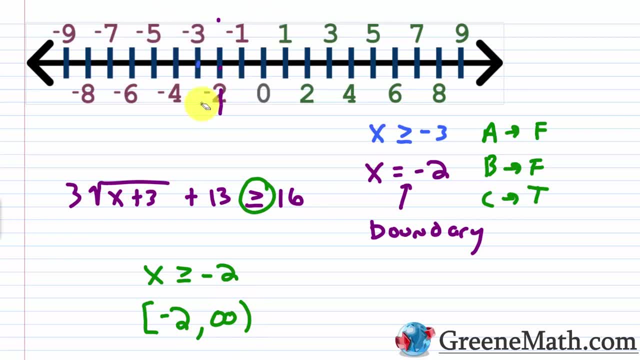 an infinity symbol and a parenthesis, And then graphically you can kind of follow that Same pattern. We'll put a bracket at negative 2. And we'll just shade everything to the right. Okay, And that'll be our solution. 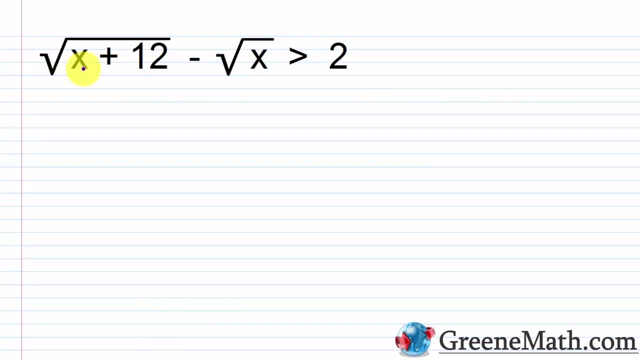 All right, Let's take a look at another one. So we have the square root of x plus 12 minus the square root of x is greater than 2.. So since we have two square roots involved, we're going to think about two different domain restrictions. 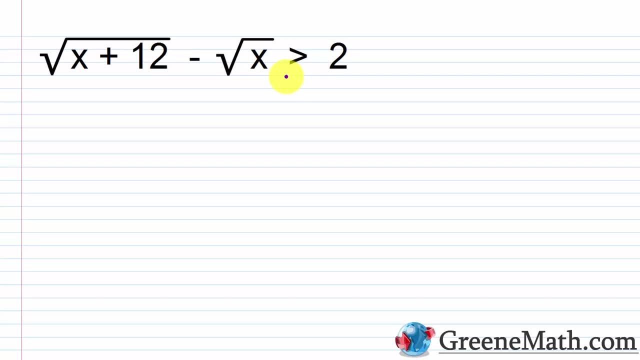 And we got to go with the stricter one, Okay. So for this one I would set x plus 12 and say that's got to be greater than or equal to 0.. And then for this one, I would say x has to be greater than or equal to 0. 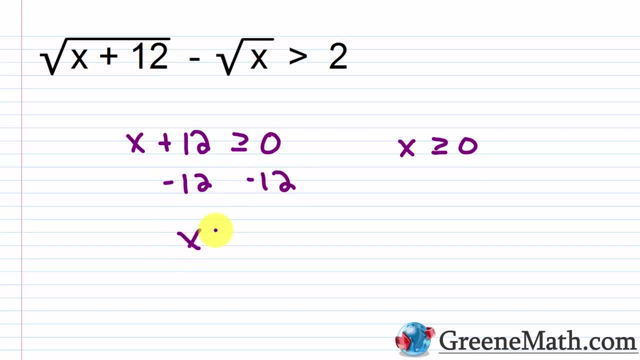 So for this one, I subtract 12 away from each side. I find that x has to be greater than or equal to negative 12.. For this one, we know that x just has to be greater than or equal to 0.. This one is more restrictive. 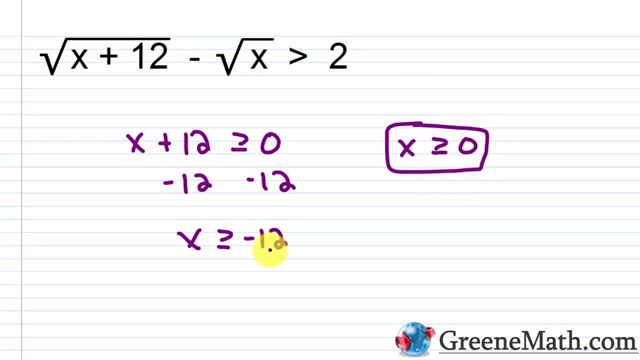 Okay, So I'm going to go with this one as my domain, Because if I got a value that's between negative 12 and 0, it wouldn't work Right. It might work in this one, but it's not going to work in that one. 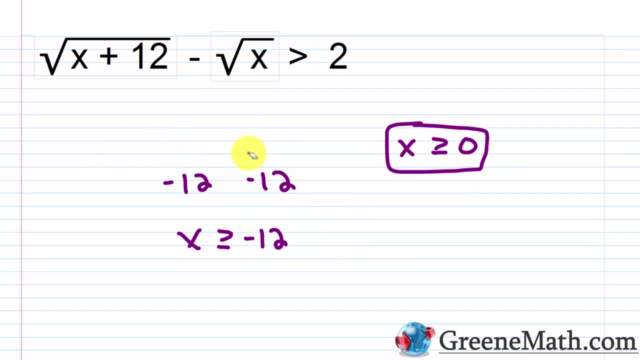 Okay, So you've got to go with the stricter one. So what we're going to say is that x has to be greater than or equal to 0.. So let's just write that over here. We'll say: x has to be greater than or equal to 0.. 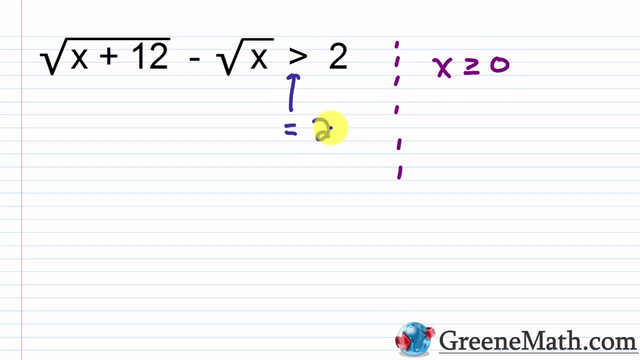 All right, Now to solve this, I'm just going to replace this with equals, So I'm going to have the square root of x plus 12 minus the square root of x is equal to 2.. All right, So I'm going to isolate one of the radicals. 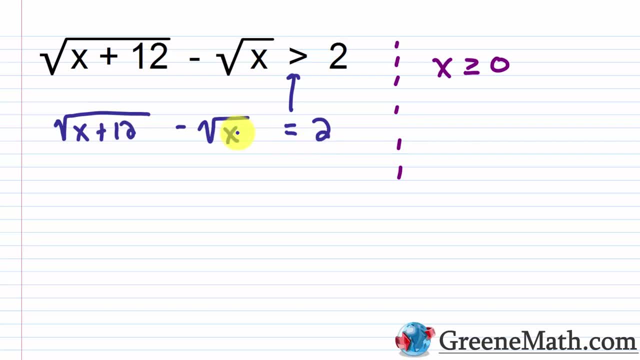 I have two involved, So you can isolate either one first. It doesn't matter, It's probably going to be easier to isolate this one. So what I'm going to do is I'm going to add the square root of x to both sides of the equation. 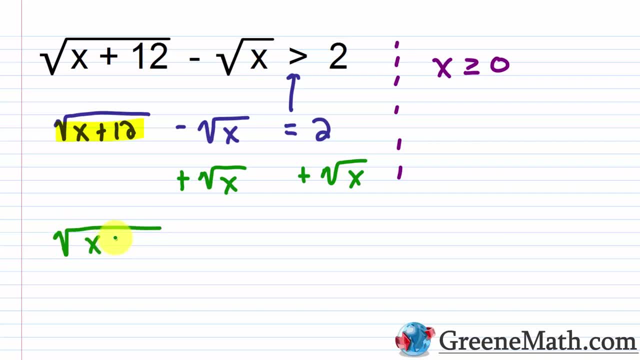 And so on the left, I'm going to have the square root of x plus 12. And this is going to be equal to: on the right, I'm going to have the square root of x and then plus 2. So now I'm going to square both sides. 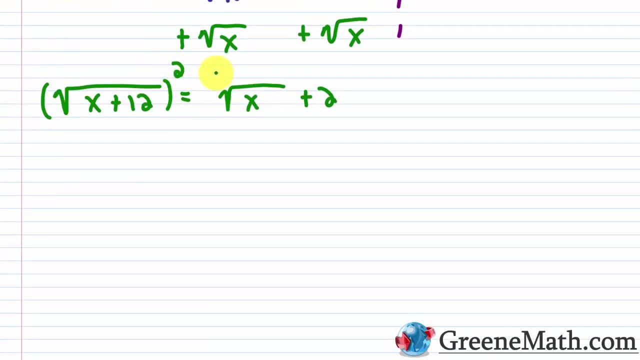 Let me get some room going. I'm going to square this side and I'm going to square this side. So on the left I'll just have x plus 12.. On the right, remember, I have to expand this, So you can use FOIL or you can use your special products formula. 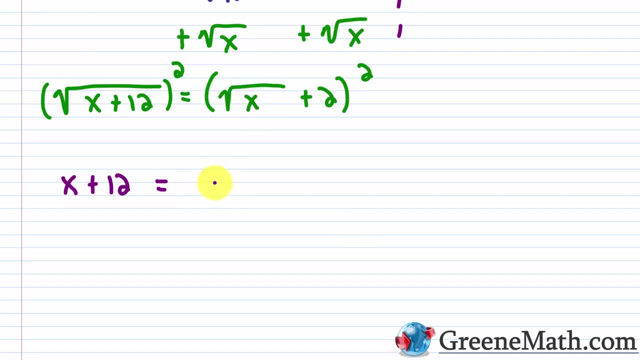 So I would square this first guy. So the square root of x squared is x, And then plus you'd have 2 times this guy times this guy. So 2 times 2 is 4.. Then times your square root of x. 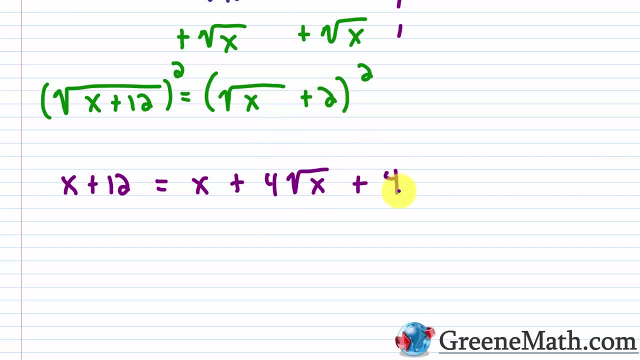 Then, plus the last guy, 2 squared, which is 4.. So I still have a radical involved. So I need to make sure that I clear that guy out. So I want to isolate that again. So what I'm going to do first is just kind of simplify or clean things up. 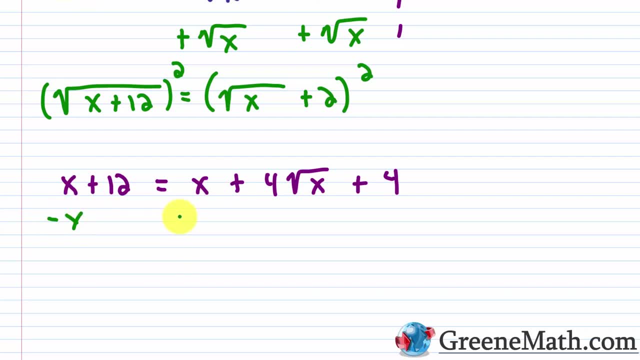 I have an x on each side. If I subtracted that away from each side it would cancel everywhere, And basically what I'm going to do is subtract 4 away from each side. So I'm going to have that 8 is equal to 4 times the square root of x. 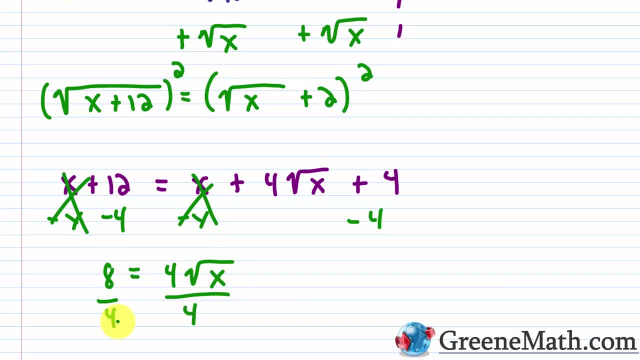 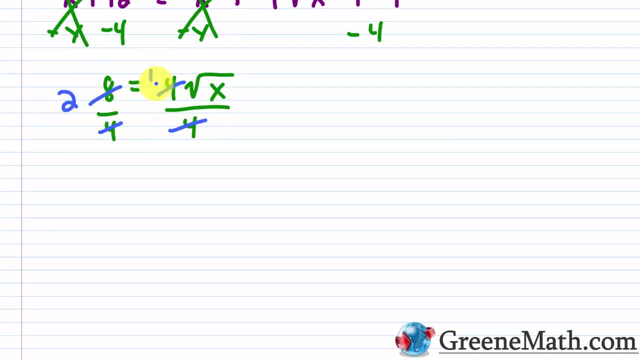 Again, if I want to isolate the radical, let's divide both sides of the equation by 4. And let me kind of get some more room going. So this cancels with this and gives me a 2.. This cancels with this and gives me a 1.. 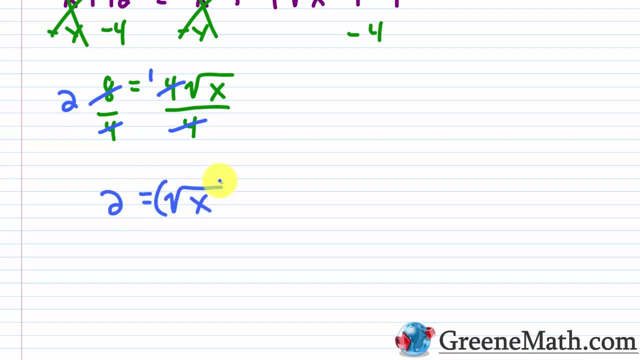 You've got: 2 is equal to the square root of x. If we square both sides, we're going to get that 4.. 4 is equal to x. Okay, or x equals 4.. So let me erase everything, All right. so we found that our boundary was x equals 4.. 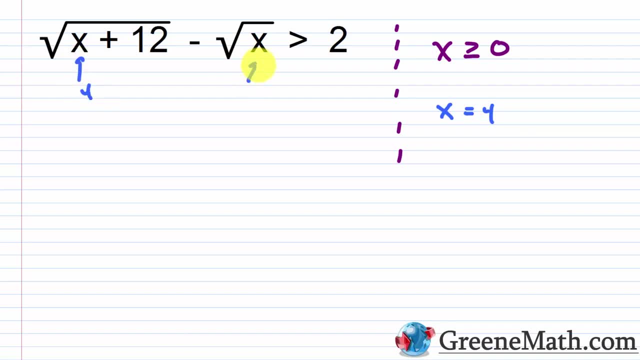 Again, you can check this If you plug in a 4 there and there, 4 plus 12 is 16.. Square root of 16 is 4.. Then minus the square root of 4 is 2.. Again, I replace this with equals. 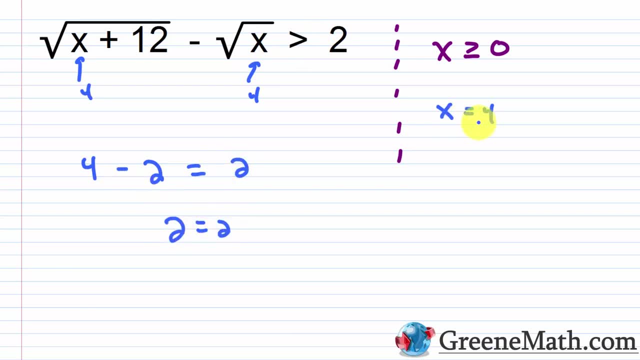 So 4 minus 2 is 2.. 2 equals 2.. So that works out right. We don't have an extraneous solution Now. this is a strict inequality. So 4 does not work as a solution. Okay, so we know that. 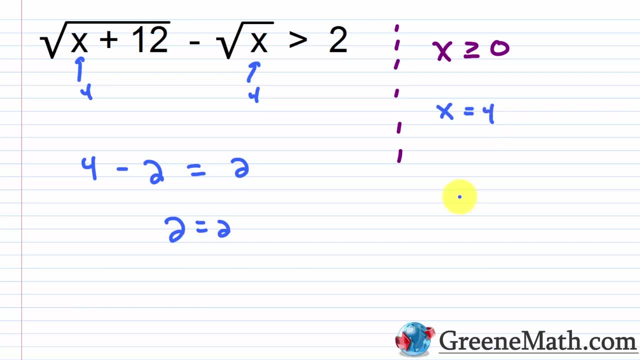 What we want to do is go to the number line and we want to test values on each side of 4 to see what works and what doesn't. Now we know that we have a domain restriction here, that x has to be greater than or equal to 0. 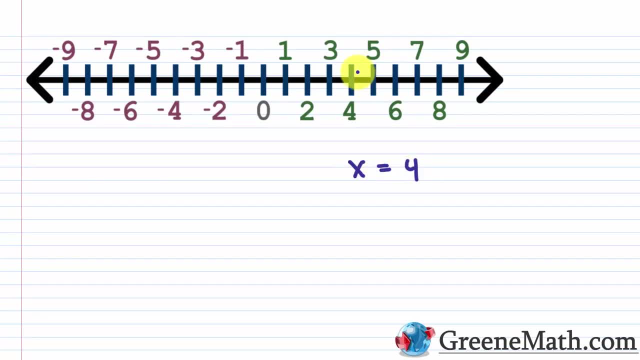 All right. so we found that our boundary was at x equals 4.. All right, so here's 4 on the number line. So I want to test values on each side of this, But remember x needs to be greater than or equal to 0.. 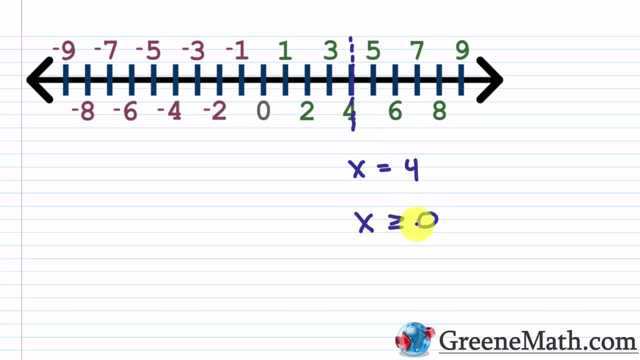 This is our domain restriction. So if I test values on the left side of 4, what would I get? So let's go ahead and rewrite our inequality, So we have the square root of x plus 12 and then minus the square root of x. 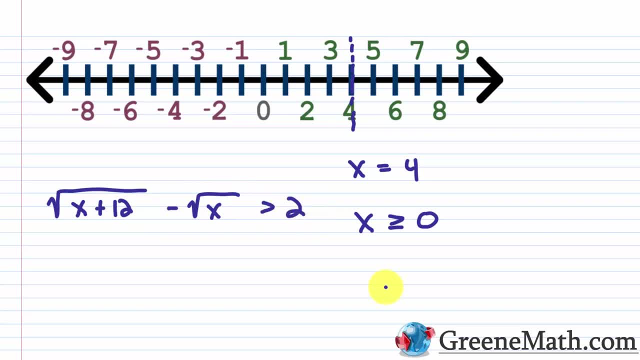 And again, this was greater than 2. So I can choose anything I want, with the exception that it has to be greater than or equal to 0. Right, so it's got to be kind of to the right or equal to that 0 there. 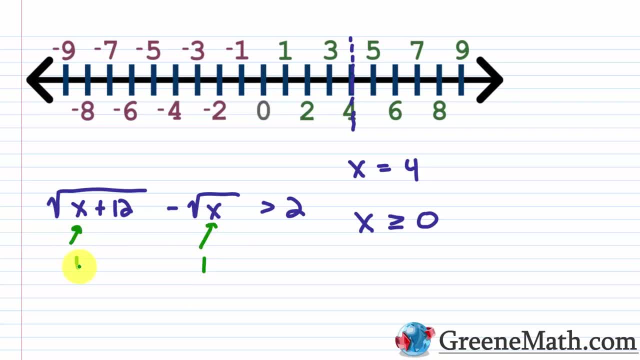 So let's just go ahead and pick 1.. So if I plugged in a 1 there and there, what would I get? Well, here on the left, you'd have square root of 1 plus 12, which is square root of 13.. 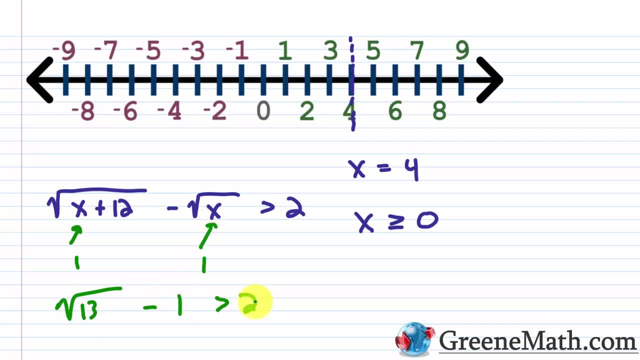 Then minus square root of 1 is 1.. This should be greater than 2.. So the square root of 13 is about 3.6.. Okay, if I subtract away 1, you'd have about 2.6.. 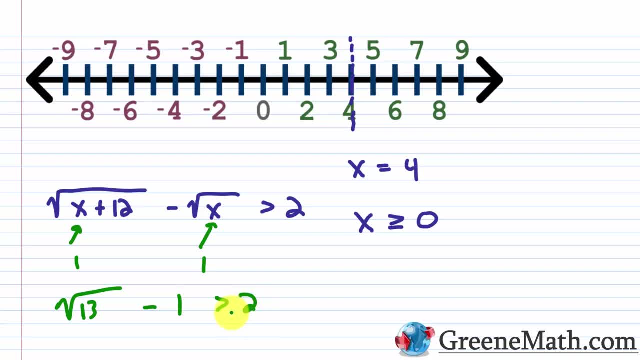 So that would work. That would be greater than 2.. So basically, values to the left of 4 work, with the exception of they have to be greater than or equal to 0. So we can say that anything. let's call this interval a. 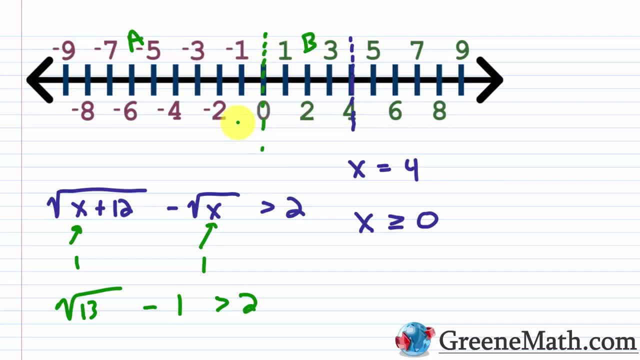 Let me kind of divvy this up And let's call this, Let's call this interval b. So anything in interval a, that's to the left of 0, doesn't work right because it violates our domain. Then anything in interval b is going to work right. 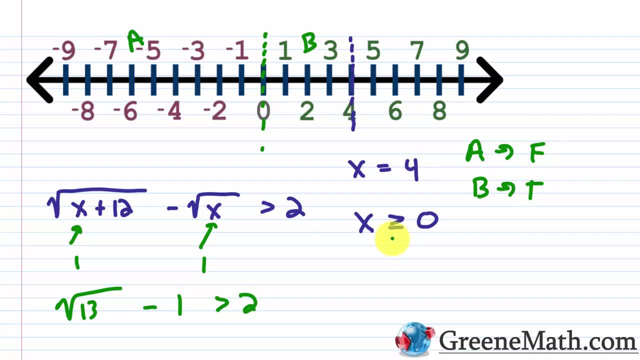 because it's greater than or equal to 0, but less than 4.. So that's going to be good to go. What about anything in interval c? So that's going to be anything that's larger than 4.. So let's test that out. 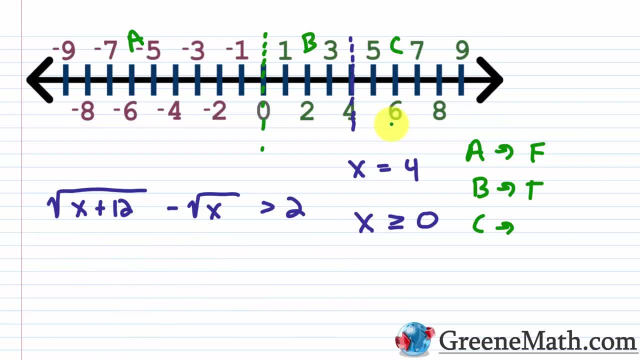 Let's erase this, And I can check a value over here. Let's just choose the value 9.. Plug that in there and there. So 9 plus 12 is 21.. So you'd have the square root of 21.. 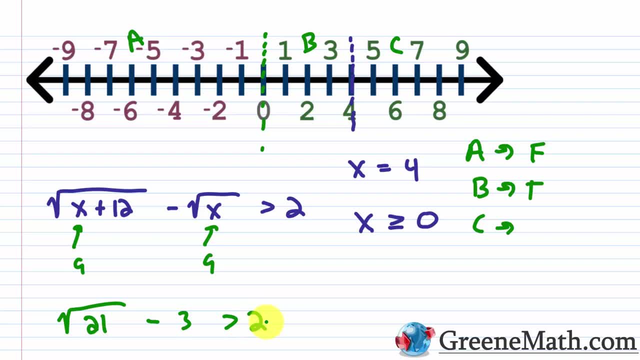 Then, minus The square root of 9 is 3.. Is that greater than 2?? Well, the square root of 21 is about 4.58.. OK, that's an approximation. If I subtracted away 3,, I'd have about 1.58.. 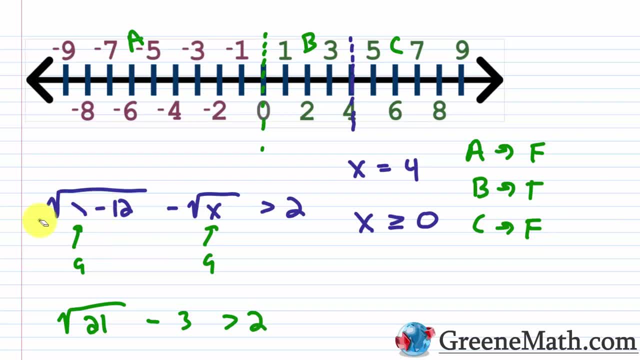 So that's not greater than 2.. So this would be false. So we have our solution here. We found that values in interval b will satisfy the inequality, So essentially it's anything that includes 0. Up to, but not including 4.. 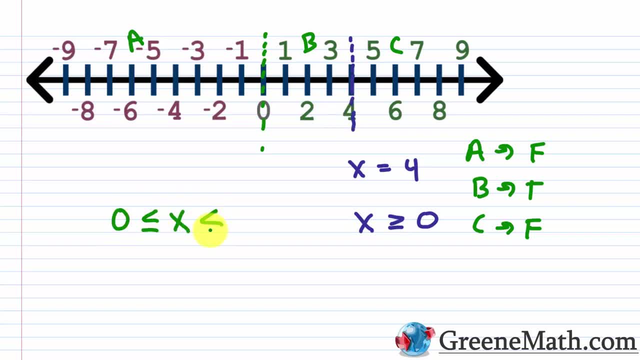 So x can be greater than or equal to 0 and less than 4.. OK, anything in that range. In interval notation again, you put a 0 next to a bracket and then a 4 next to a parenthesis, And then graphically, OK, graphically. 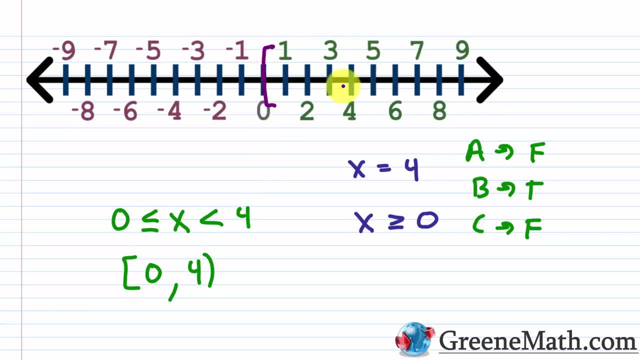 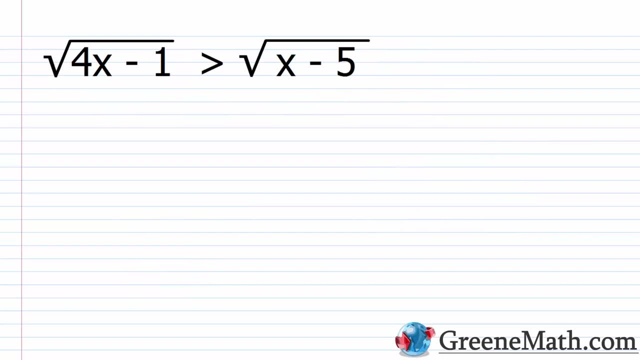 we would put a bracket at 0 and we put a parenthesis at 4 and we would shade everything in between. All right, let's take a look at the next example. So we have the square root of 4x. So we have the square root of 4x minus 1 is greater than the square root of x minus 5.. 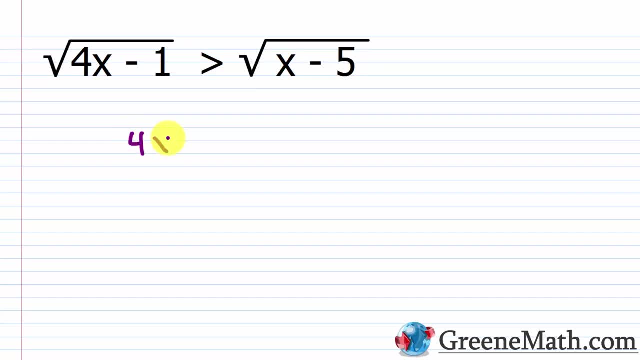 So for this guy again, I've got two domain restrictions that I need to consider. I've got that 4x minus 1 has to be greater than or equal to 0. And let's do that first. So let's add 1 to each side of the inequality. 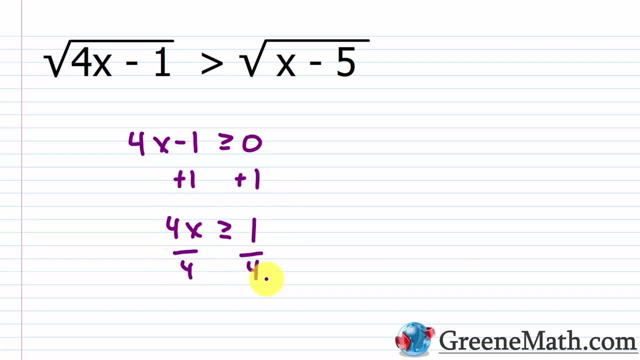 You'd find that 4x is greater than or equal to 1.. Divide both sides of the inequality by 4.. You'd find that x has to be greater than or equal to 1 4th. So here this one's going to be more restrictive, right. 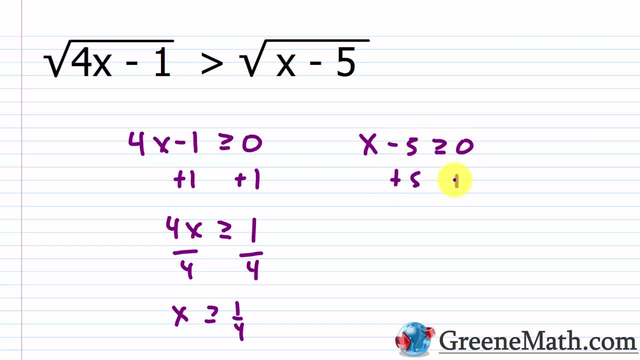 4x minus 5 is greater than or equal to 0.. I add 5 to both sides of the inequality. I find that x has to be greater than or equal to 5.. So again, this one's more restrictive. So that's going to be our domain. 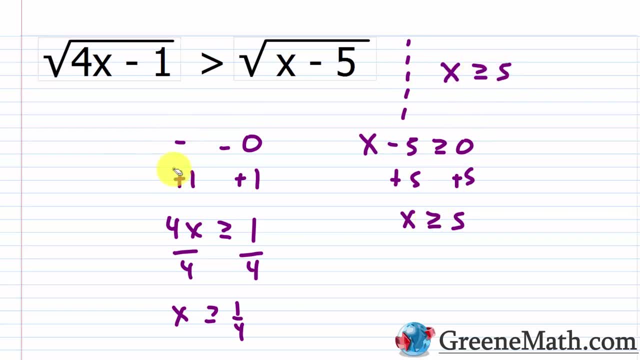 So x has to be greater than or equal to 5.. OK, let's erase all this now that we know what we're looking for, And let's replace this inequality with an equals, So we would have: the square root of 4x minus 1 is equal to the square root of x minus 5.. 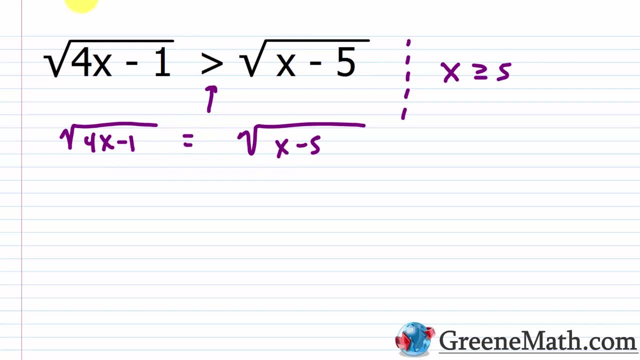 Let me make that a little better. So both radicals are isolated here. So let's just square both sides And I'll have my. 4x minus 1 is equal to x minus 5.. Let's add 1 to both sides of the equation. 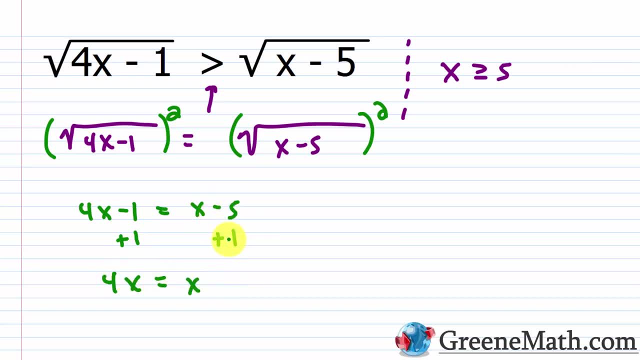 You'll get that 4x is equal to x, And then negative 5 plus 1 is going to be negative 4.. Let's subtract x away from each side of the equation. We're going to do this over here. We'd end up with: 3x is equal to negative 4.. 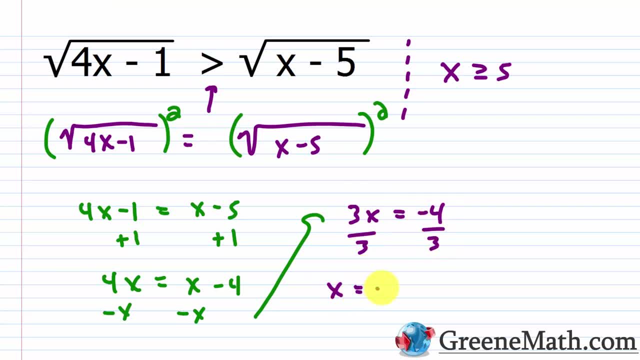 Divide both sides of the equation. Divide both sides of the equation by 3. You get: x is equal to negative 4 thirds. OK, so let's erase this. So what happens is this guy is extraneous And you can immediately see that it's not going to work if you plug it in here. 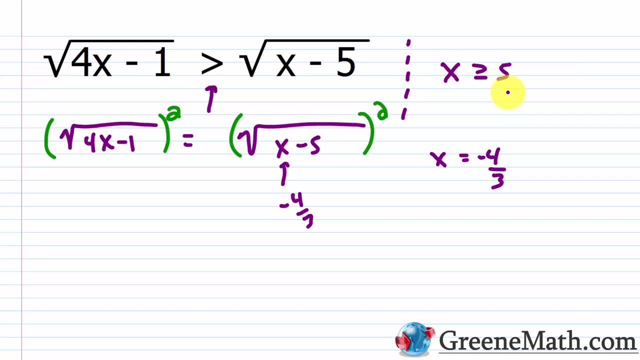 Because it's going to violate your domain. x has to be greater than or equal to 5. So you can kind of get rid of this. at this point A lot of people would stop and say, OK, well, there's no solution. 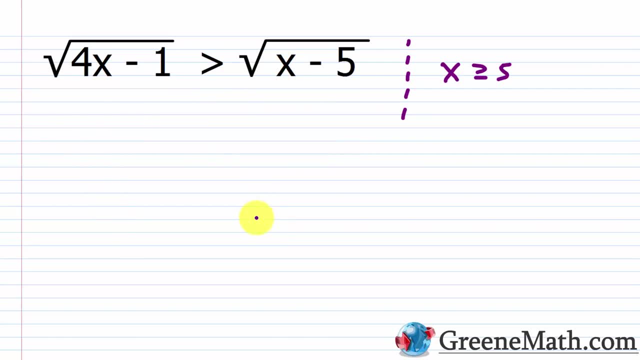 But that's not actually true either. So here's where you've got to kind of go down to the number line and consider things. So we know that. We know that this guy is only valid for values of x that are greater than or equal to 5.. 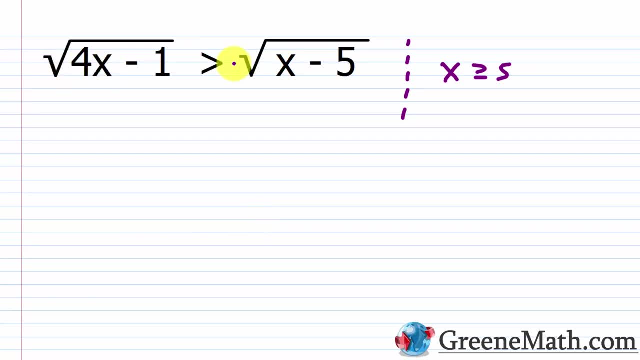 But I want you to think about something. You have the square root of something And then you have the square root of something. You're saying: where is the square root of this expression greater than the square root of this expression? Well, if I'm doing the same thing to each side again, you could just consider where. 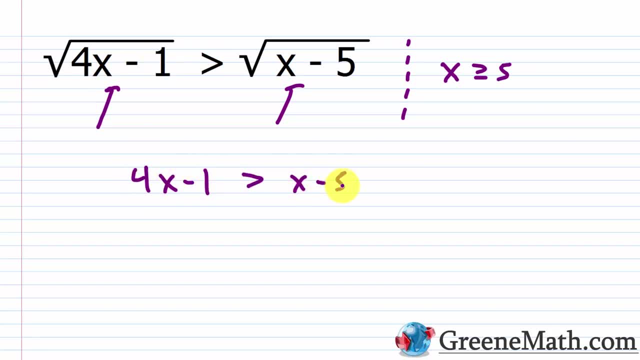 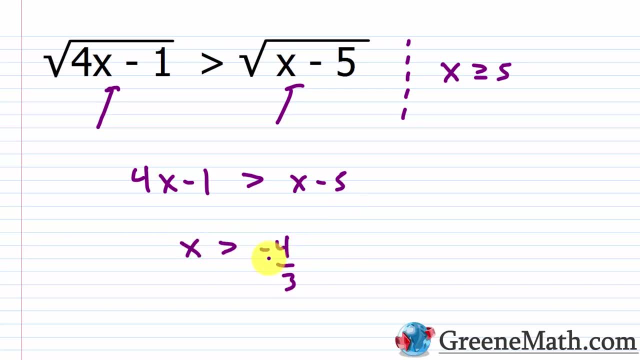 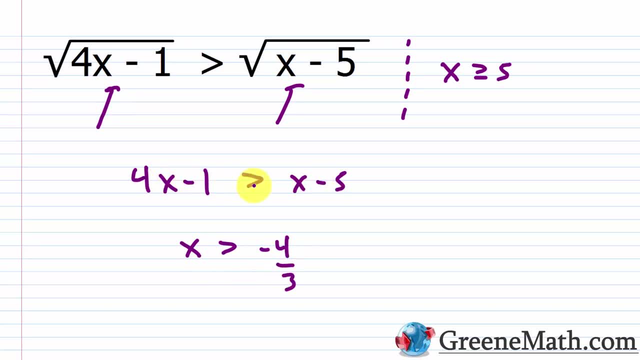 side here is less than the left side, where you can say the left side is greater than the right side. Okay, So that means that for values where it's valid, in the domain where x is greater than or equal to 5, the left side should be greater than the right side. 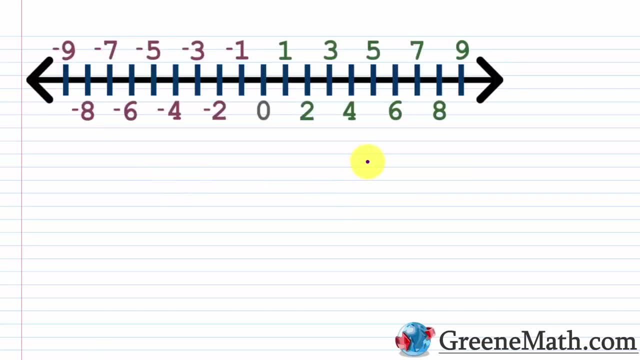 So we can check that. Let's go down to the number line And again the domain here is that x, x is greater than or equal to 5.. So at 5, I'm just going to put a little border And I'm going to say that we can test something to the right of 5.. 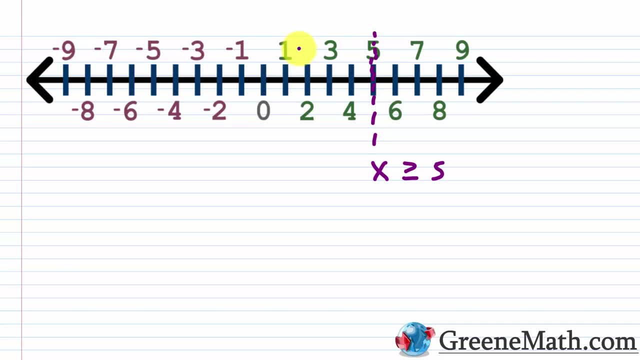 We know, anything to the left of 5 doesn't work because it violates the domain. So I'll call this interval a and this interval b And I'll say that in interval a nothing works. okay, because it violates the domain. So for interval b I can just choose something. 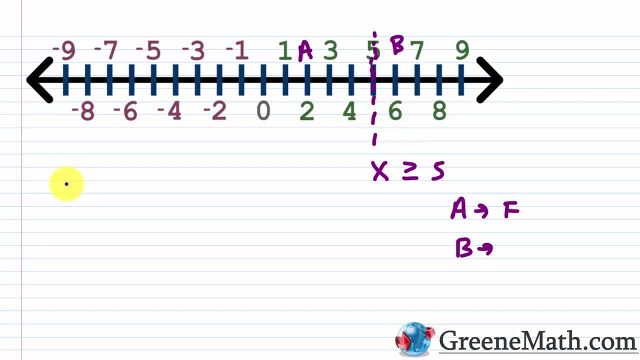 Let's just choose something like 6, and we can check that. So remember we had that the square root of 4x minus 1 is greater than or equal to negative 5.. So what's the square root of 5?? 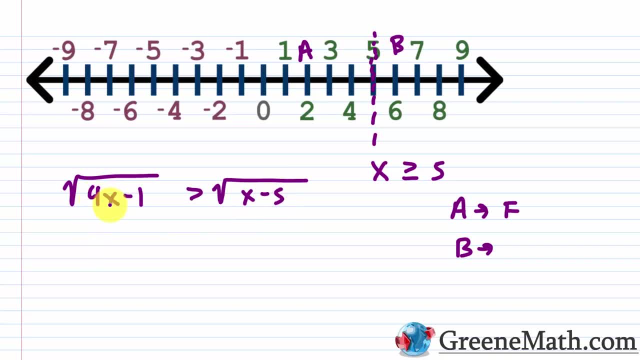 Well, the square root of 5 is greater than the square root of x minus 5.. If I plug in a 6 for x, I'd have 4 times 6,, which is 24,. 24 minus 1 is 23.. 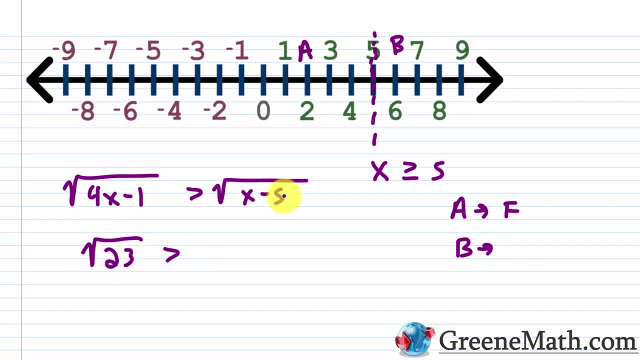 So the square root of 23 is greater than 6 minus 5 is 1,. square root of 1 is 1,. okay, So what's the square root of 23? if I approximate that, Well, it's going to be about 4.79, so that's clearly greater than 1.. 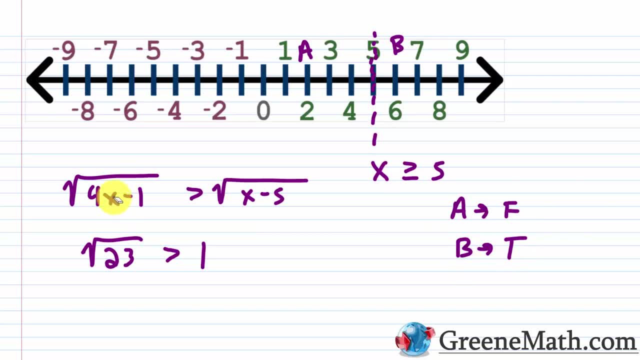 So in this interval b, things are going to work. okay, So this is going to be our solution. It's basically that x is going to be greater than or equal to 5, okay, So we'll say x is greater than or equal to 5.. 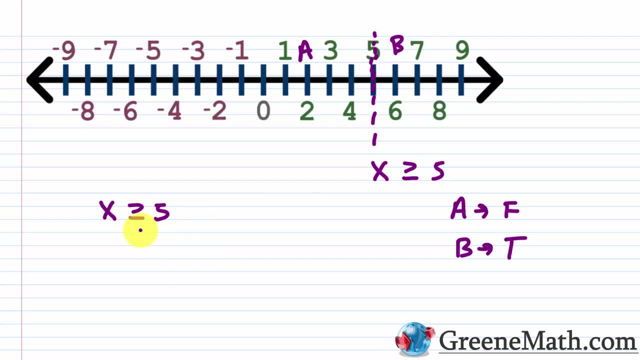 That's both our domain restriction and our solution for the inequality. And graphically I can just put a bracket at 5 and just shade everything to the right. In an interval notation I can put a bracket, a 5, comma and then infinity, okay. in a. 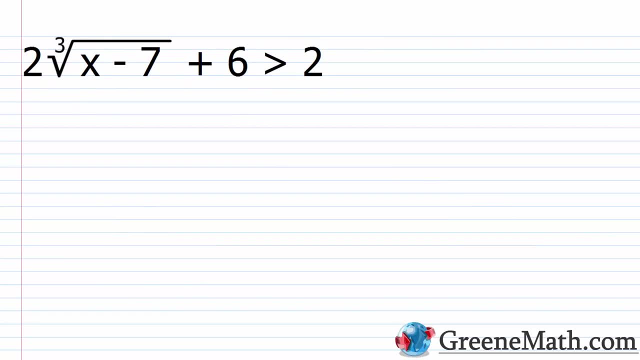 parenthesis. All right, let's look at one with a cube root involved, So these are a lot easier. When you have a cube root, you don't have a domain restriction, so I don't have to start by saying x minus 7 is greater than infinity. 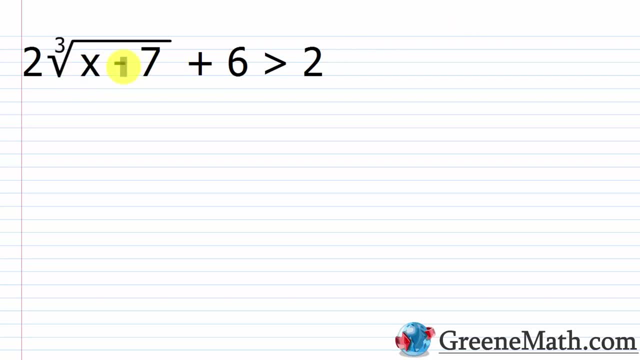 Let's say x minus 7 is equal to 0. This value, here, this radicand, can end up being whatever. okay, It can be negative, It can be 0.. It can be positive. Remember, in the real number system you can take the cube root of a negative number. okay. 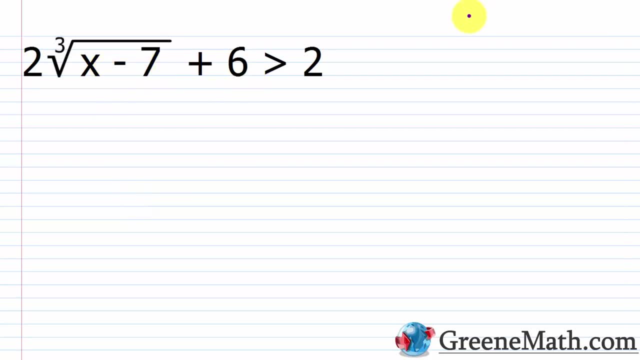 So you're good to go there. So all I'm going to do is just solve this guy. Let's go ahead and replace this guy with an equals and solve So 2 times. the cube. root of x minus 7 plus 6 is equal to 2.. 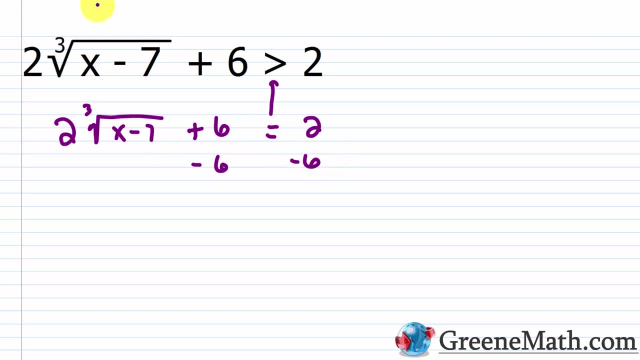 Let me again isolate the radical. so let me subtract 6 away from each side of the equation. That'll cancel. You have 2 times the cube root of x minus 7 is equal to negative 4.. Let me divide both sides by 2 so I can isolate the radical. 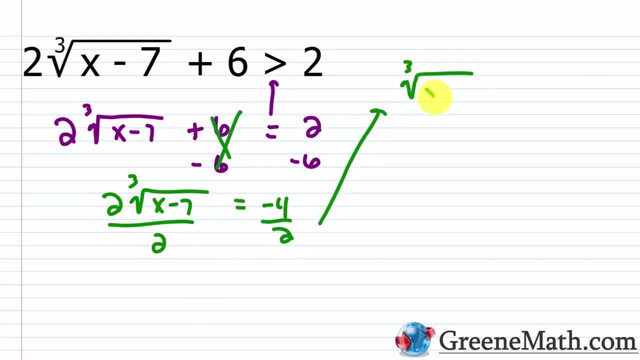 Let me kind of move this up here. You'll have the cube. root of x minus 7 is equal to negative. 4 over 2 is negative 2.. So to get rid of the radical, I'm going to cube both sides of the equation and I'm going 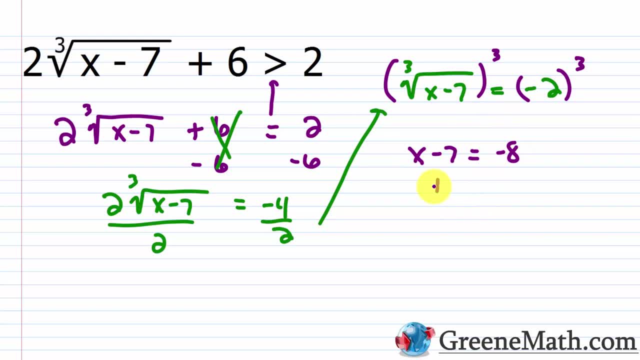 to find that x minus 7 is equal to negative 8. Let me add 7 to both sides of the equation and I'll find that x is equal to negative 1. So again, that's the boundary. So let me erase all this. 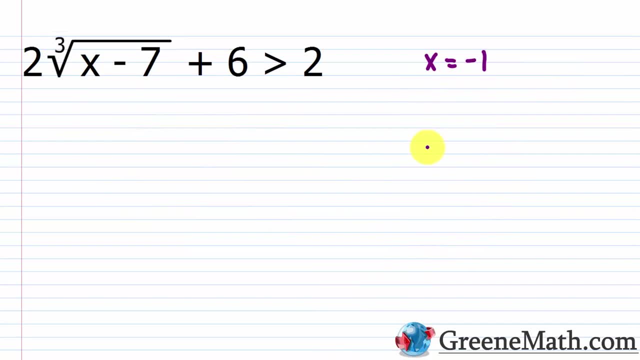 x equals negative 1.. Again, that's the boundary And I don't have a domain restriction, So let me go down to the number line. So here's negative 1.. So basically, you're going to have two scenarios. You're going to have this interval a and this interval b. 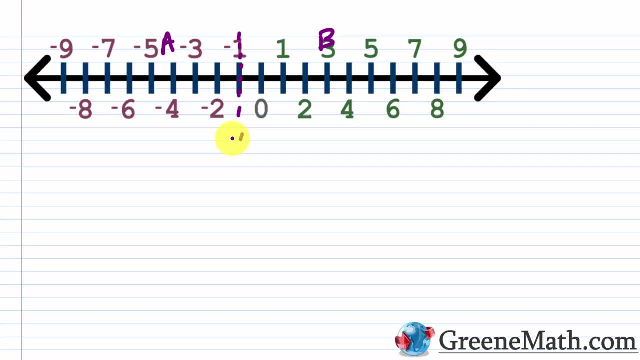 You don't have any domain restrictions, So just pick something in interval a and test it. So again, we have 2 times the cube root of x minus 7 plus 6, and this should be greater than 2.. Okay So, 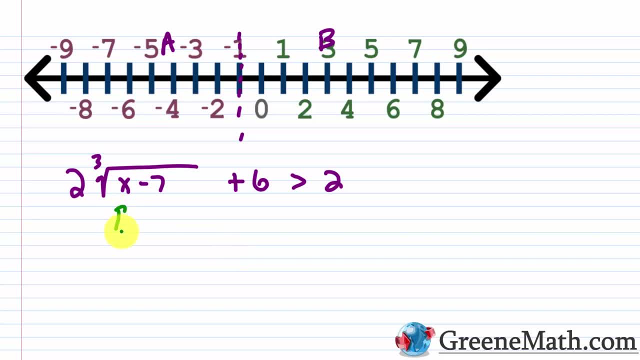 So the cube root of negative 1, we can pick, let's say, negative 20.. So negative 20 minus 7 is negative 27.. So the cube root of negative 27 is going to be negative 3.. So 2 times negative 3 is negative 6.. 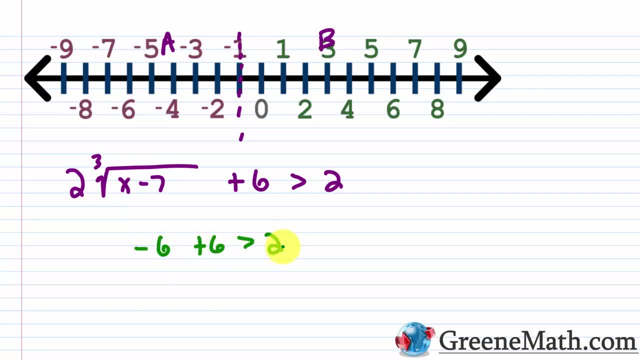 So you'd have negative 6 plus 6 is greater than 2, which is false. So I know values in interval a don't work. So this is going to be false. Then what about values in interval b? So let's choose 8.. 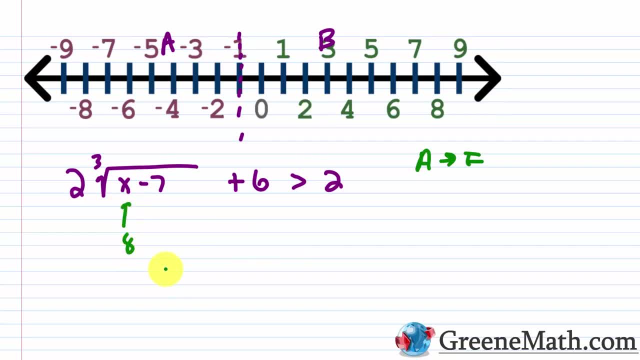 So I'll plug in an 8 there. 8 minus 7 is 1.. Cube root of 1 is 1.. So 2 times 1 is 2. Plus 6 is greater than 2.. You get 8 is greater than 2, which is true. 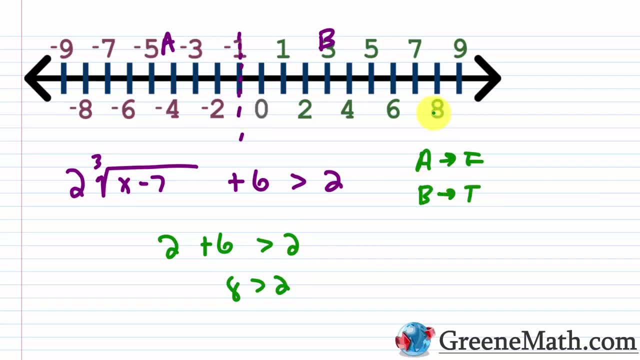 So for interval b, it's true. So anything larger than negative 1 would work. So we can say our solution here is that x is greater than negative 1.. Alright, So in interval notation you've got negative 1 comma infinity Again, with a parenthesis next to each. 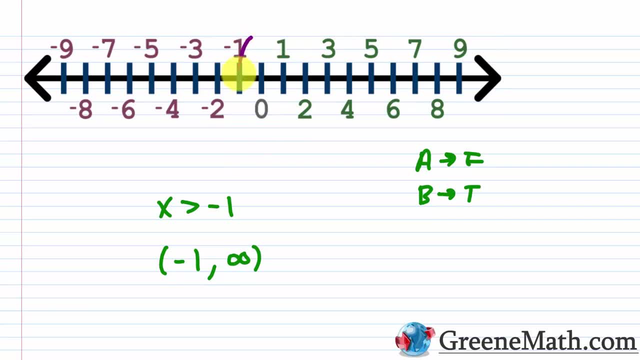 Let me erase this Graphically. I'm going to put a parenthesis at negative 1. I'm just going to shade everything going to The right And then heading right, maybe to the middle here, To the right, And then from there it'll go to the back. To the left, Right To the back, And then pin is added. in That way it'll be indicated. I'll go right at that moment, right here, And we're going to put the table here. So what's the difference between negative and positive plates up? And then entered total weight And then it's going to go to the right, Okay, And then가� бр Mary IV is negative, So the parentheses have to be bald or heavily Said, because i'm impressed that the part Simply So, and let me know what you think and what's going to happen. If it's negative, then i'm going to go with negative, but I suggest that it's going to be electric, Okay, great.